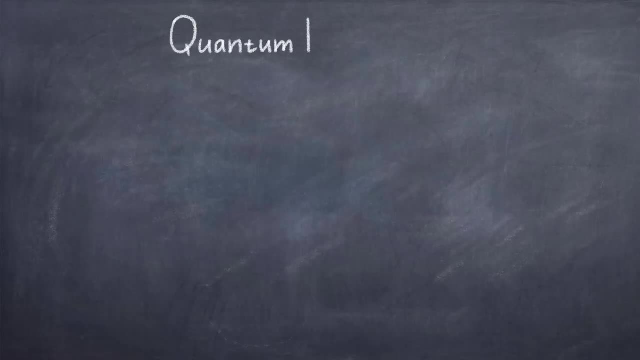 In this video we will take a deeper look at the weak force. The theory behind this force is called quantum flavor dynamics or QFD, because this force can change the flavor of particles. What we mean about changing flavor is changing the identity of a particle. Two examples of flavor: 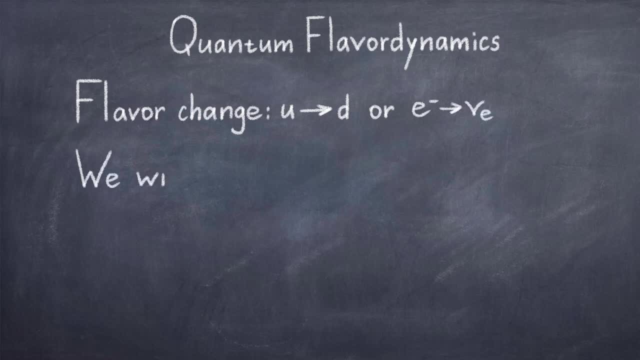 change is when an up quark is changed to a down quark and when an electron is changed into a neutrino. It is, of course, not possible to change particles arbitrarily, as barrier, number, charge and color must be conserved, so there are some rules this force must abide to. In this video we will 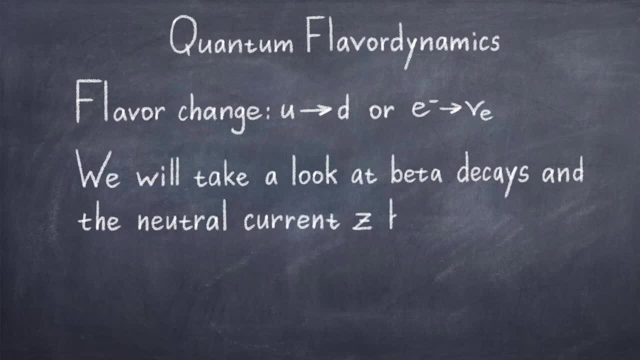 take a closer look at the processes caused by the weak force, such as the very important beta decays and the neutral current diagram which led to the discovery of the C boson. We will also discuss why the range of this force is so short. The fact that the range is so short is also why we can't really experience it in the same way as 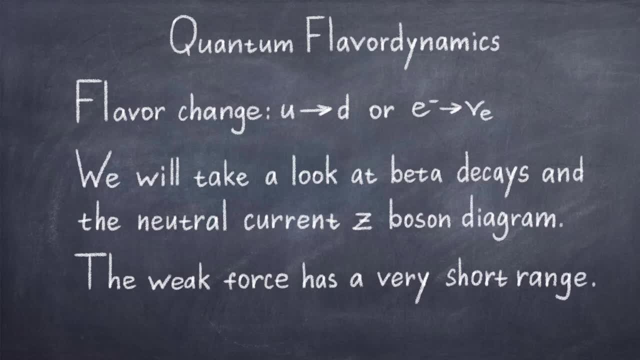 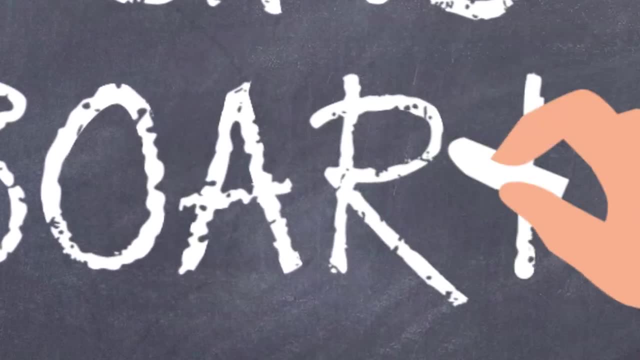 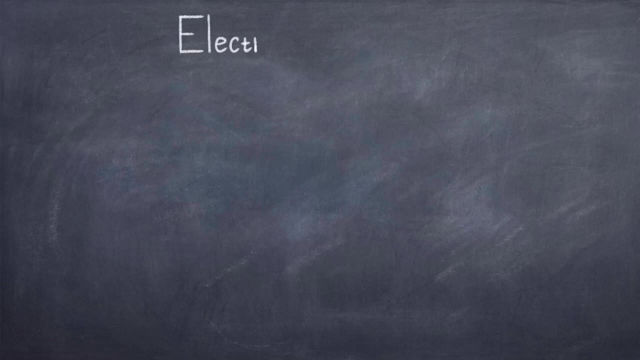 the electromagnetic force or gravity, which technically have infinite ranges. In the video about QED, we started by looking at the Lagrangian of QED. This is, however, not really possible for the weak force, and this is related to fact that the fundamental symmetry of the weak force is more complicated. 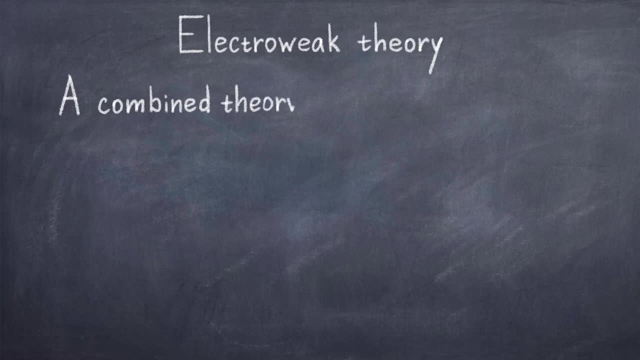 To understand the weak force in terms of Lagrangian, one would need to consider electroweak theory, which is the combined theory of the weak force and electromagnetic force. In fact, this electroweak theory contains all the information of the weak force and 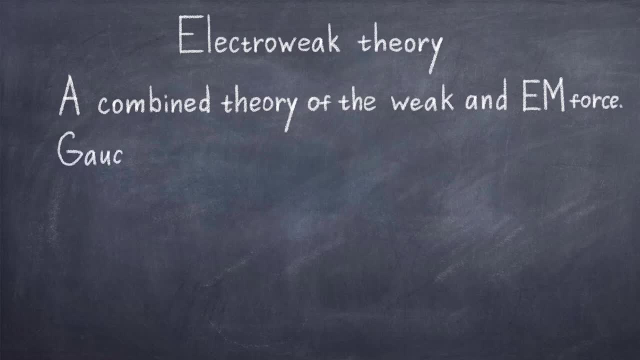 the electromagnetic force combined. The simple way of explaining why you cannot write a Lagrangian for the weak force in a similar way to the electromagnetic force is because of gauge invariance. We discussed this a bit in the video about fundamental forces, but the essential part 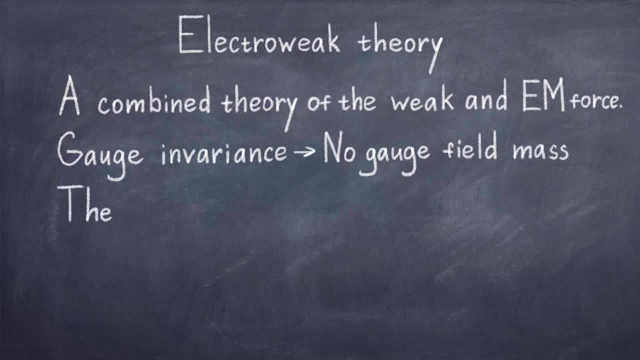 is that to keep gauge invariance means that you are not allowed to have explicit mass terms of your gauge field, or in other words, your force carriers must be massless. The difference between QED and the weak force is that the QED boson, the photon, is massless. 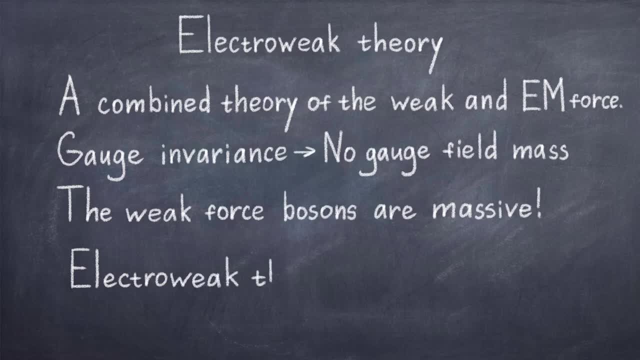 but the weak force is massless. QED boson is massless. The weak force bosons are all massive. so if you want to see the details of the theory behind this force, then let me know and we can take a deeper look at the electroweak theory. 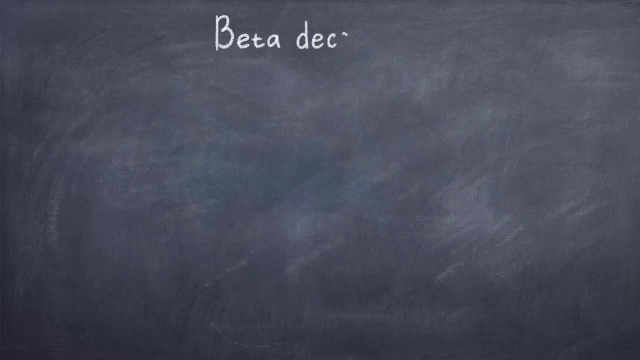 The weak force is most famously known for being the force behind beta decays. Beta decays are when unstable atoms send out high-energy electrons or positrons as radiation in order to eventually reach a more stable state. There are two types of decays. 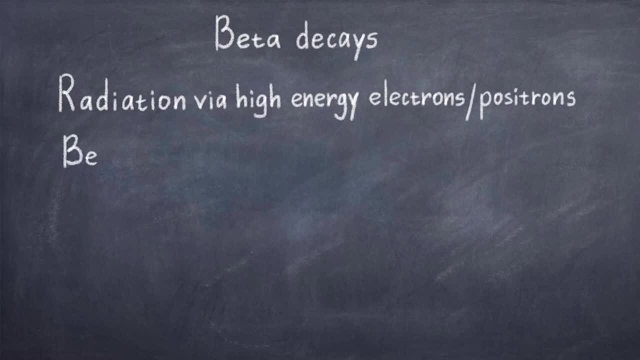 Beta plus and beta minus decay. This sign refers to the charge of the particle. thus, the beta minus decay is when an electron which has a negative charge is emitted. Likewise, a beta plus decay is when a positively charged positron is emitted. 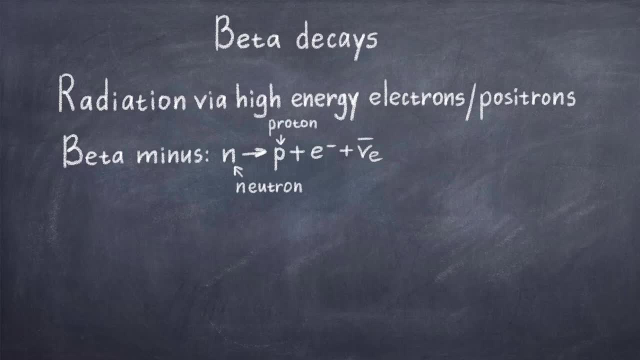 We can write the process of a beta minus decay in the following way, where a neutron N turns into a proton P plus an electron and an anti-electron neutrino. Likewise, A beta plus decay can be written as a proton P turns into a neutron N plus a positron plus. 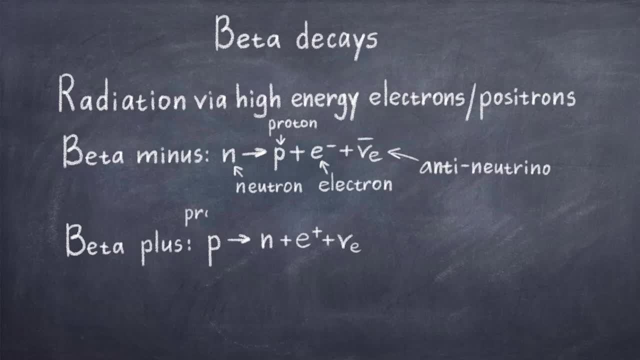 an electron neutrino. Note that these neutrinos are necessary to conserve lepton numbers. This we discussed in the video about particle physics. This process is very important in nuclear physics and the decays of unstable atoms. It is fundamentally caused by the weak force. 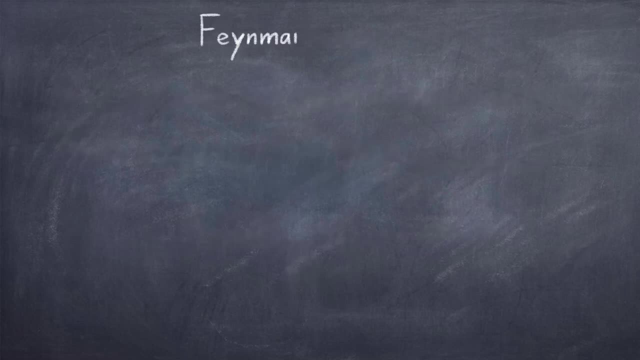 To understand exactly what is going on in these beta decays. I will show you how to do it. Let's dive in deeper. We will now look at the beta minus decay. but the principle is exactly the same for the beta plus decay, just the particles are a bit different. 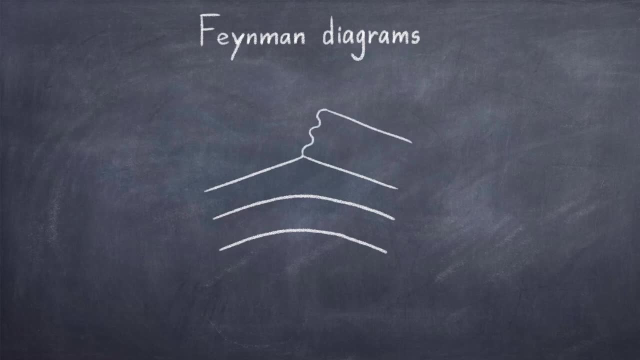 The weak force is emitted by three particles: the W minus, W plus and the C bosons. The two W bosons are the particles behind beta decays And the negative discharge is in the beta minus decay and the positive discharge is in the beta plus decay. 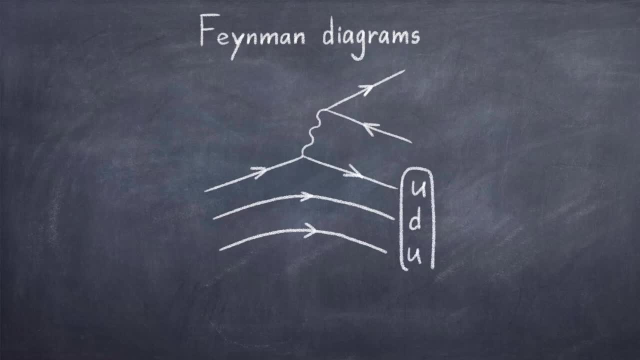 Let us write the Feynman diagram of the beta minus decay to illustrate exactly how the weak force makes this decay happen via the W minus boson. First we have a neutron which is changed into a proton via a W boson. Because the neutron is neutral and the proton has a plus one charge, we must have the negatively. 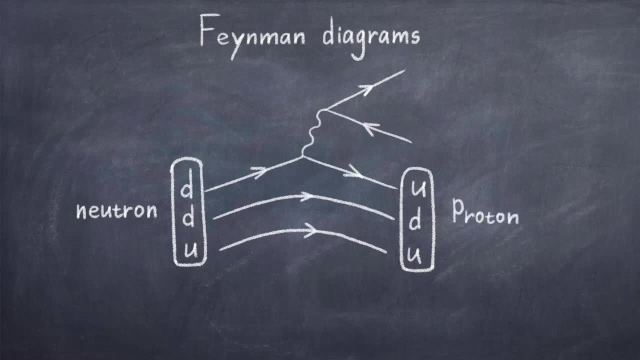 charged W boson such that the resultant charge is zero, just like the neutron, which started the process. Now the proton continues its life as usual, but the W boson has a very short lifetime and quickly decays into an electron and an electron antineutrino. 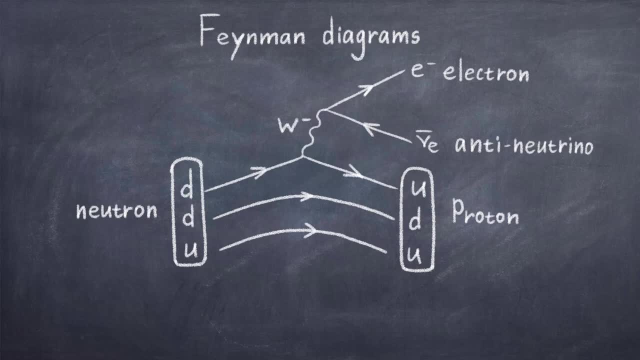 Note again how the negative charge of the W boson is given to the electron, Because neutrinos are neutral and very hard to detect. we never notice them in our everyday life. Thus, if we measure this process from a radioactive substance, the Geiger counter will just measure. 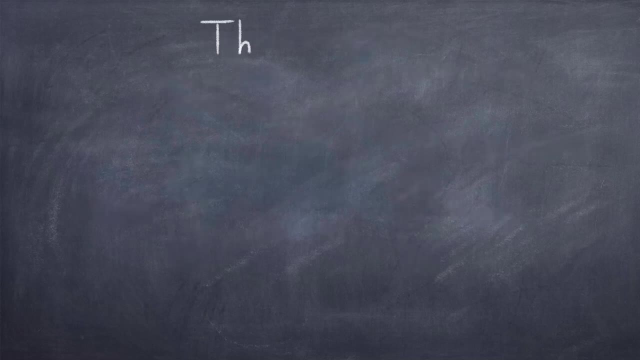 how many electrons are produced. The weak force is also mediated by the neutral Z boson. This boson is effectively like a heavy photon. By this I do not mean that you can see it as light, but from the point of view of interactions. 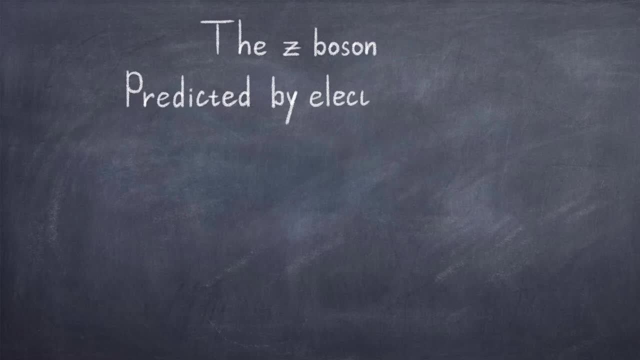 it is very similar Because the weak force interacts with all fermions and because the Z boson is neutral. one can take all possible diagrams of QED and then replace the photon with a Z boson. but because this boson is much heavier, it takes more energy for these processes to 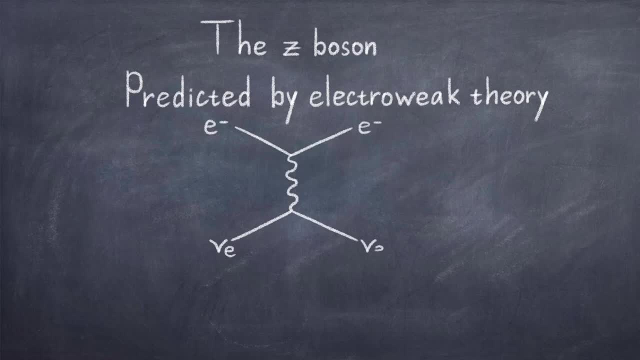 take place, and that is why they are rare. This boson was predicted by the fundamental electroweak theory. Now, unlike the photon, the Z boson interacts with the neutrinos, and neutrino interactions are a bit of a signature of the weak force, because it is the only force to interact with. 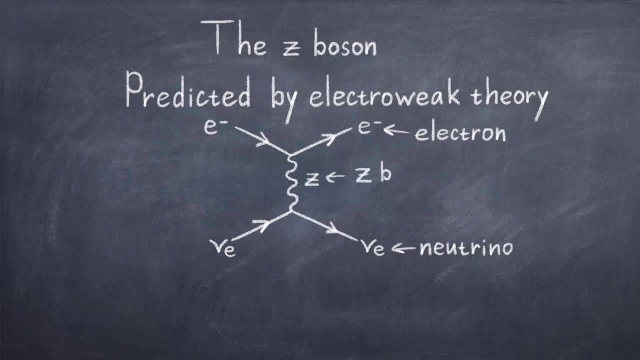 neutrinos. Because the Z boson interacts with both electrons and neutrinos, one can have scattering between the two. Thus an electron can scatter off a neutrino via a Z boson. This was how this boson was detected in 1973.. 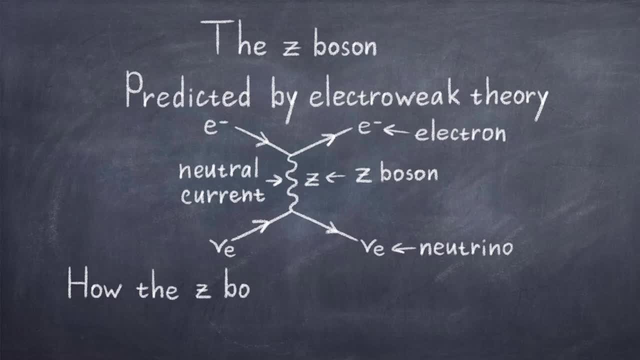 Scientists measured that the electrons suddenly moved in their bubble chamber. It was as if they moved on their own, But they realized that actually this was exactly the predicted interaction via the Z boson. Neutrinos are everywhere in the universe, but we can hardly detect or feel them. 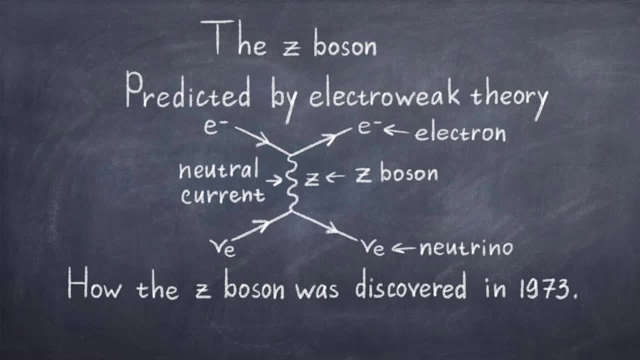 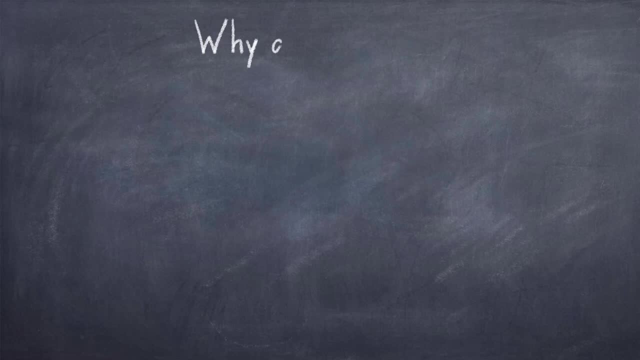 And in fact, it was these neutrinos that ever so slightly interacted with the Z boson. They could push the electrons around. Moving on with the discussion about the weak force, I would like to explain why the force is so short ranged. The key to understanding this is the uncertainty principle and the fact that the masses are. 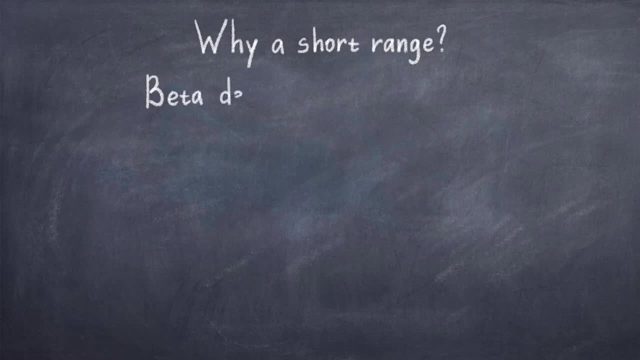 very heavy. The latter was exactly predicted to satisfy experimental results. To understand all of this, let us go back to the beta decay. Let us look at the mass situation in this simple case. So let's start with the mass. So again we have that a neutron turns into a proton plus an electron plus an anti-electron. 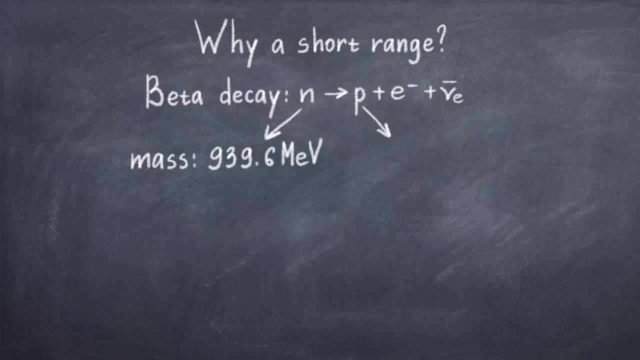 neutrino. We start with a neutron which has a mass of around 939.6 megaelectron volt. Afterwards we have an anti-neutrino which is more or less massless for all practical purposes, and the electron is so much lighter than the neutron, so its mass is insignificant. 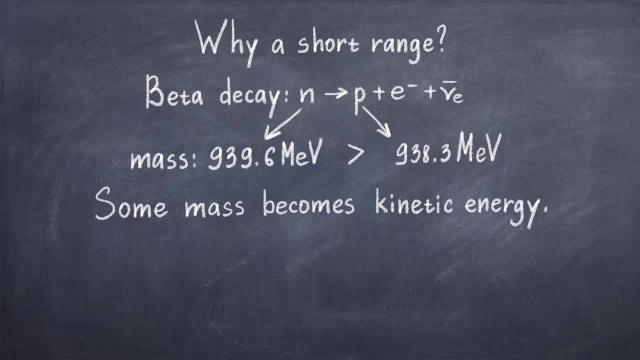 The proton, however, weighs around 938.3 MeV, Which is a bit less than the neutron. Thus, everything is fine. A bit of the mass is changed into kinetic energy, which mostly goes into the electron. So where is the problem, and what does this process have to do with the range of the weak 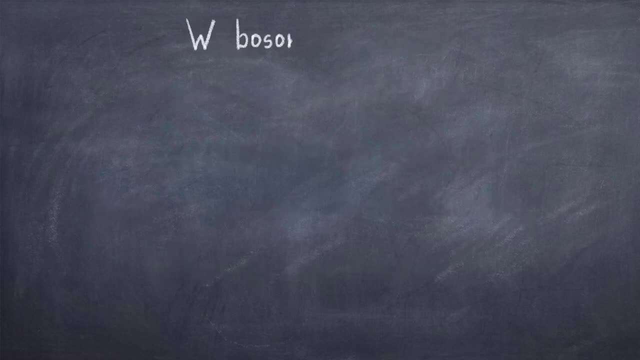 force. If we look at the process in more detail, we see that the neutron decays into a proton and a W boson. This W boson then decays into an electron and an electron anti-neutrino. So what happens? The problem is that the W boson has a mass of around 80,000 MeV, thus a bit more than 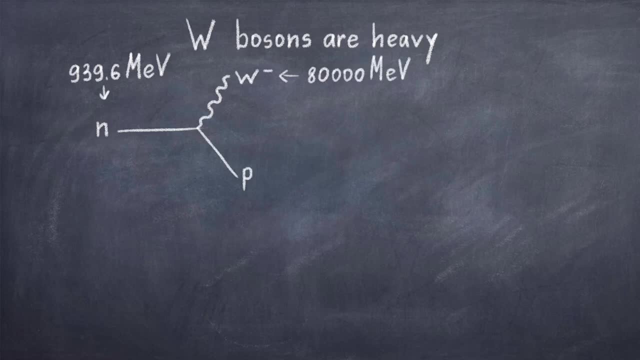 80 times the mass of a neutron, It would seem like we are creating mass out of nothing. This is where the uncertainty principle comes into the picture, Where the uncertainty in E times the uncertainty of T is greater than h-bar over 2.. 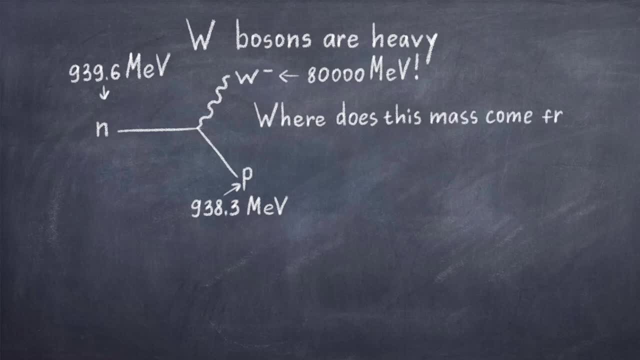